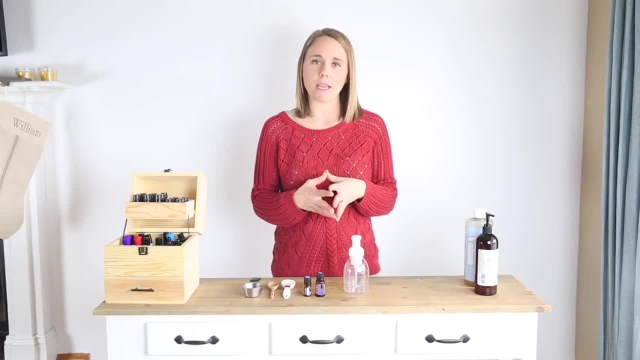 this as an all in one wash and shampoo on all of my kids and my oldest one is almost six and it still works really well for her. So this can be used for kids or babies, and I was out of it and I was getting ready to replace it and I decided I would do it here. 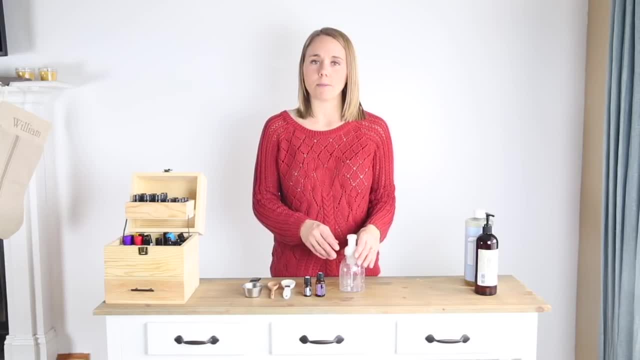 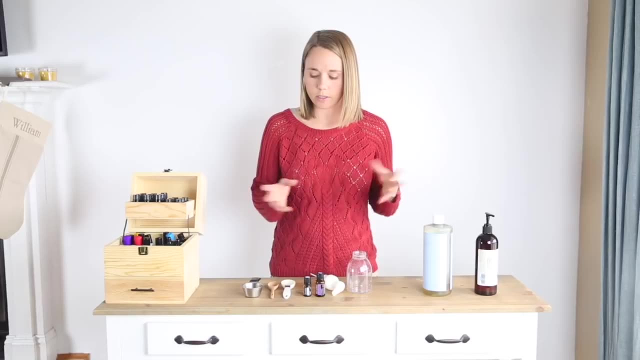 on the YouTube channel, but it almost seems silly to make a whole video for this because it is that simple to make. You only need a few simple ingredients That you probably already have in your house. It's all stuff that I have in my house. 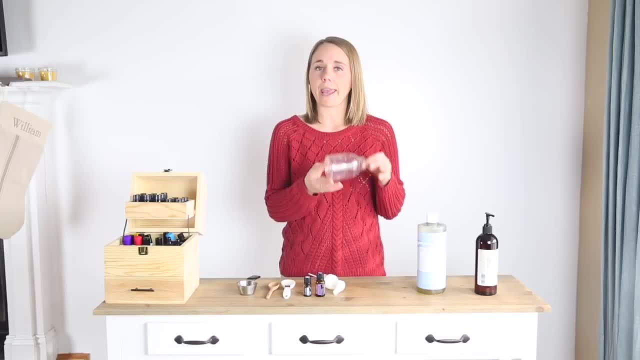 For this recipe I use a foaming hand soap container. You can use an old one that maybe you had some soap in before. You can get these on Amazon. I make a foaming hand soap for my kitchen and my bathroom, which I shared here on the. 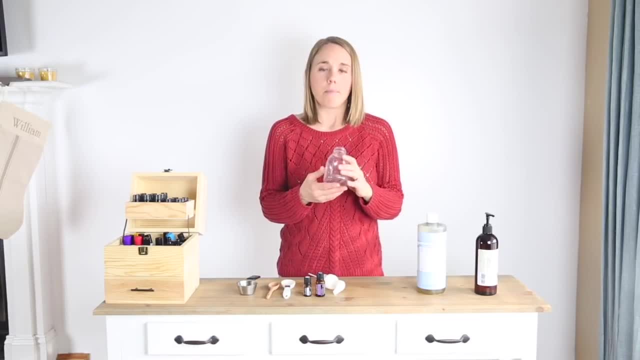 YouTube channel. I'll link that video down in the description, up in the cards. but for my kids in the bathtub I use this thicker plastic bottle and there are certain grades of plastic that are okay for baby wash. This is one of them. 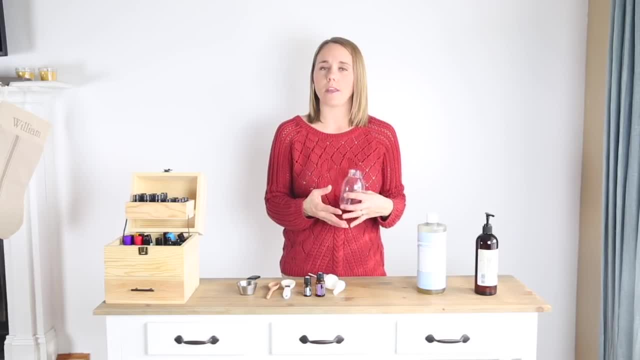 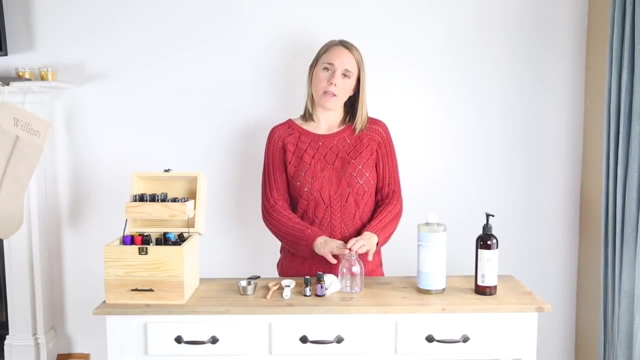 And I use that because it's in the bathtub with my kids and I don't want them to have any glass around because they would definitely break it. So I have this plastic 10 ounce foaming hand soap dispenser that I use to make this soap. 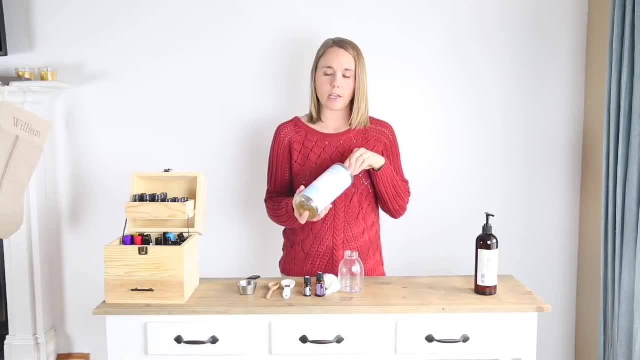 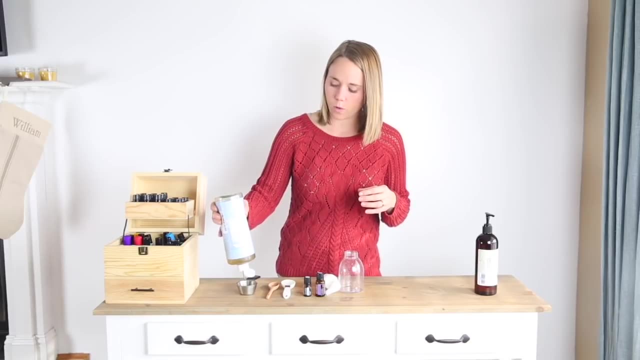 in. Okay, the first ingredient is some Castile soap. This is a very concentrated soap and it's a vegetable based soap, usually with either olive oil or coconut oil, And you're just going to use a fourth of a cup of this. 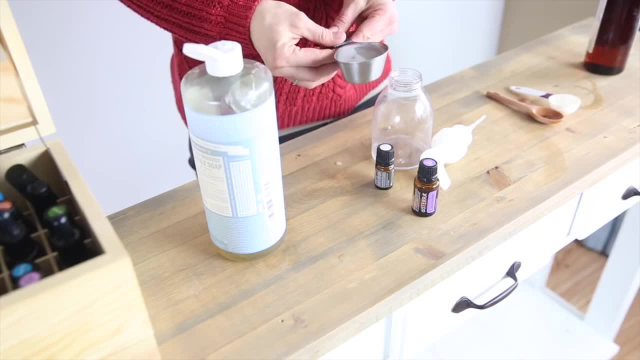 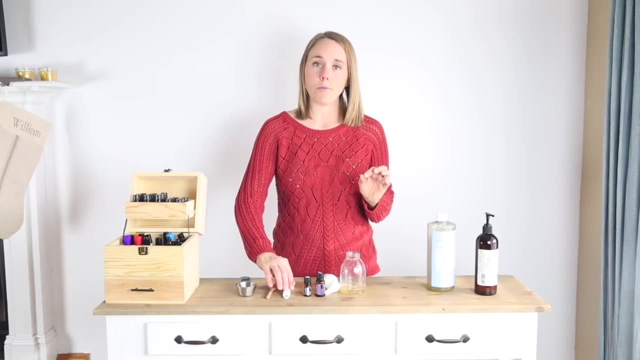 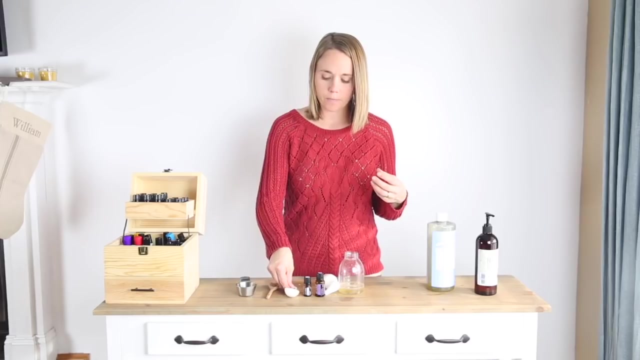 Because, like I said, it's very concentrated and a little goes a long way. So I'm just going to pour that into my soap container and then I'm going to add in a tablespoon of glycerin. Now, the glycerin helps to make this suds up and lather a little bit better. 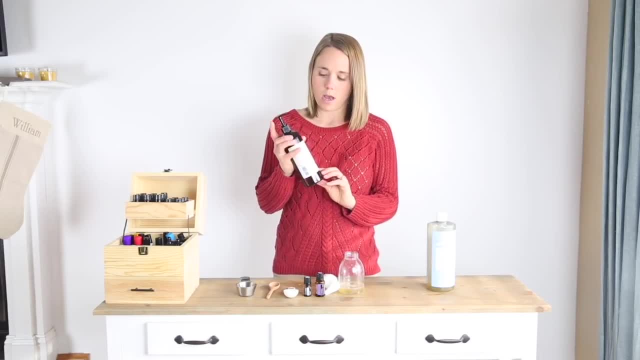 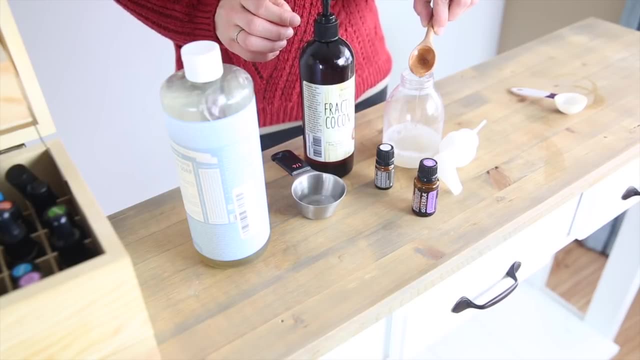 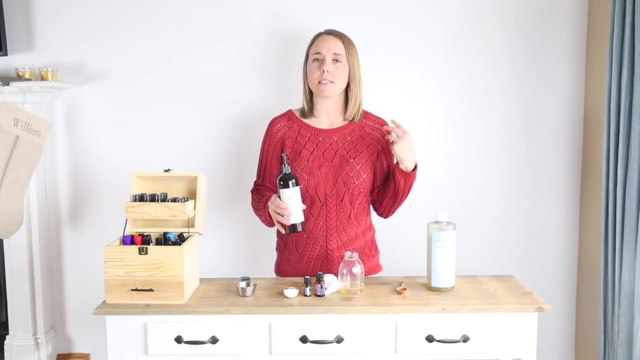 And then I'm going to add in a teaspoon of fractured coconut oil And, because I'm here making this in front of you, I'm going to measure this. but usually I just put a couple Um squirts in out of this bottle and the fractured coconut oil is going to make this. more moisturizing for your baby or child's skin. Then you can pick an essential oil or a blend of essential oils to add into this if you want it to be scented and for some extra therapeutic benefits. So the two that I have out and the two that I use most often in my baby soap is lavender. 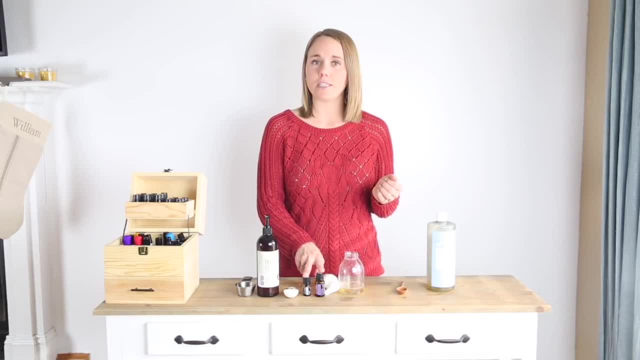 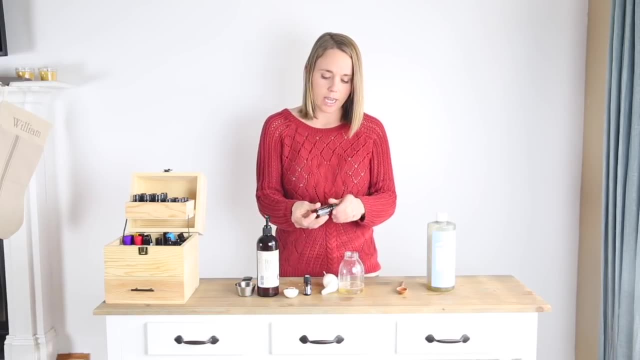 and Roman chamomile, And the reason why I use these two is because they're very calming and relaxing oils, Really gentle for delicate skin, And so I just add in about five drops of lavender, and then I'll put in about three drops of